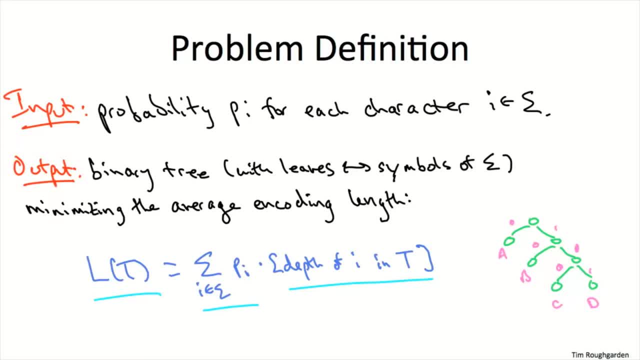 principled way, some kind of tree whose leaves correspond to the symbols of the alphabet. So let's spend a slide just thinking about. you know, at a high level, where would this tree come from? How would you build it up, given this unstructured input? 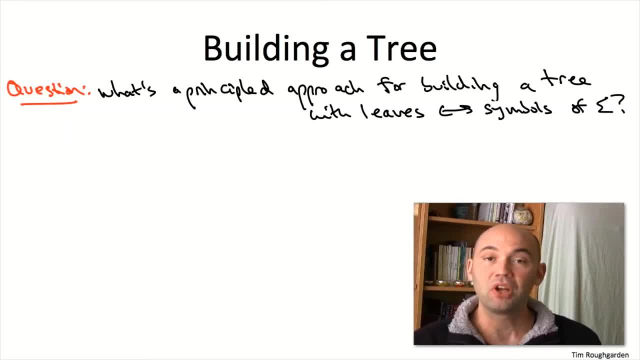 So there's certainly no unique answer to this question, And one idea, which is very natural, but that turns out to be suboptimal, is to build a tree using a top-down approach, which you can also think of as an instinctive approach. So what we're going to do is we're going to build a tree. 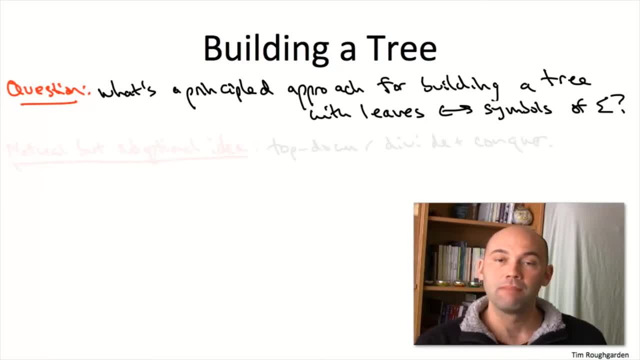 but we're also going to build a tree using a suboptimal approach. So what we're going to do is think of as an instantiation of the divide-and-conquer algorithm design paradigm. The divide-and-conquer paradigm, you'll recall, involves breaking the given subproblem into 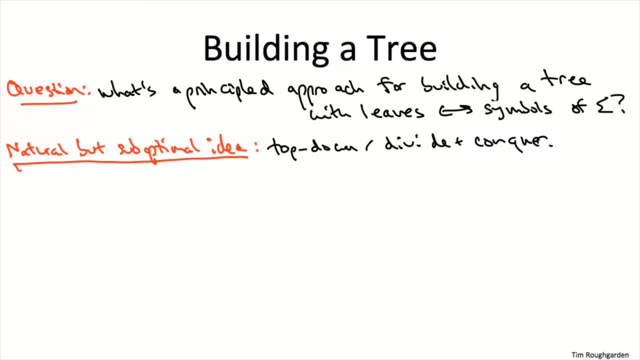 usually multiple smaller subproblems. They're solved recursively and the solutions are then combined into one for the original problem. Because trees- the desired output here- have a recursive substructure, it's natural to think about applying this paradigm to this problem. 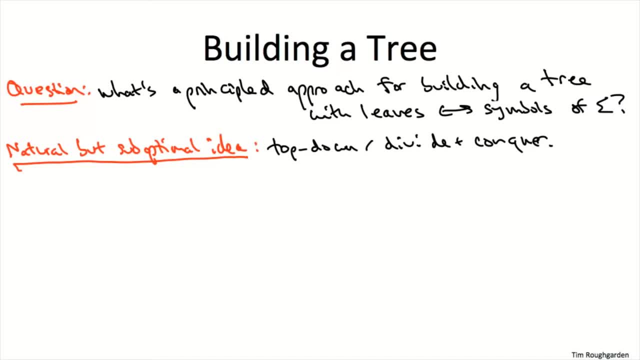 Specifically, you'd love to just lean on a recursive call to construct for you the left subtree, another subcall constructing the right subtree, and then you can fuse the results together under a common root vertex. So it's not clear how to do this partitioning of the symbols into two groups, but one idea. 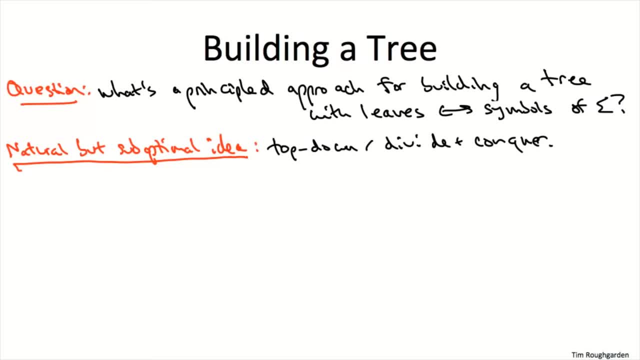 to get the most bang for your buck, the most information out of the first bit of your encoding, you might want to split them in the symbols into groups that have roughly as close to as possible of 50% of the overall frequency. So this top-down approach is sometimes called Fano-Shannon coding. Fano was a 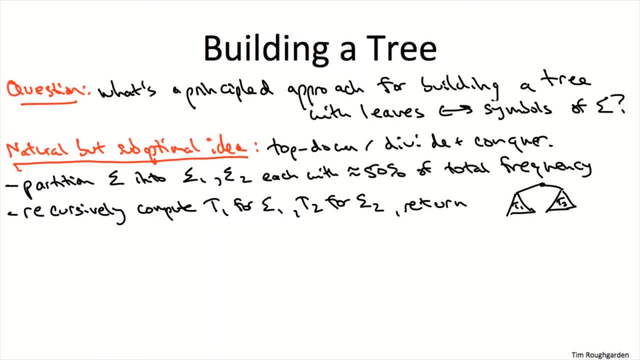 graduate advisor to Huffman Shannon is the Claude Shannon inventor of information theory. But Huffman, in a term paper, believe it or not, realized that the top-down approach is not the way to go. The way to go is to build the tree bottom-up. Not only are we going to 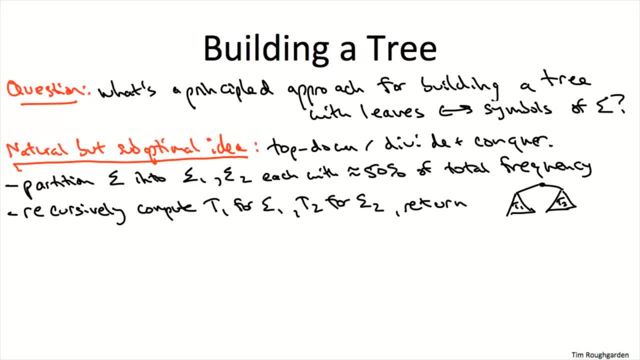 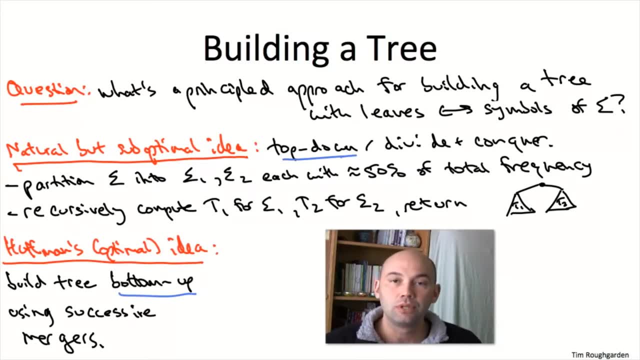 get optimal codes, but we're going to get a blazingly fast greedy algorithm that constructs them. So what do I mean by bottom-up? I mean we're going to start with just a bunch of nodes, each one labeled with one symbol of the alphabet. So, in effect, we're starting with a 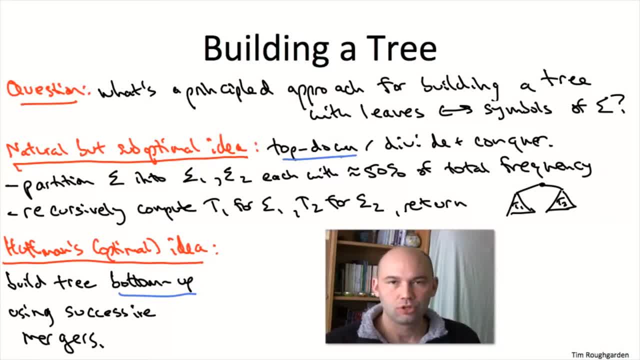 sub-tree here, which is the leaves of our tree, and then we're going to do successive mergers. We're going to take at each step two sub-trees thus far and link them together as sub-trees under a common internal node. So I think you'll see what I mean in a picture. 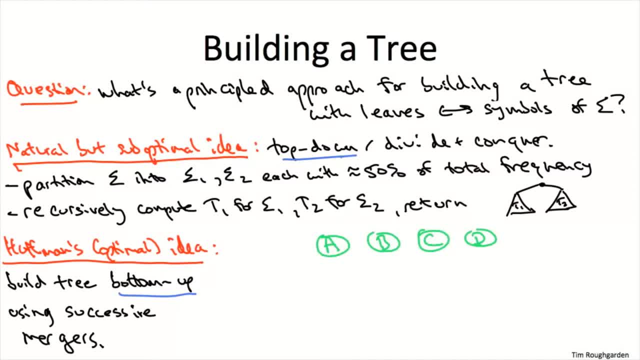 So imagine we want to build a tree where the leaves are supposed to be just A, B, C and D, So one merger would be: oh well, let's just take the leaves C and D and link them as siblings under a common ancestor. 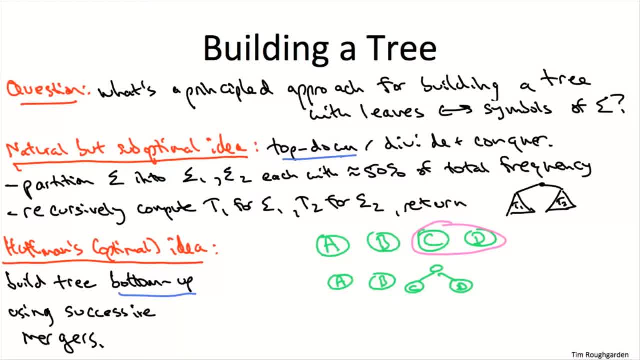 leaf B with the subtree we got from the previous merge, The subtree comprising the nodes C, D and their common ancestor. So now, of course, we have no choice but to merge the only two subtrees we have left, and then that gives us a single tree, which is in fact exactly the same. 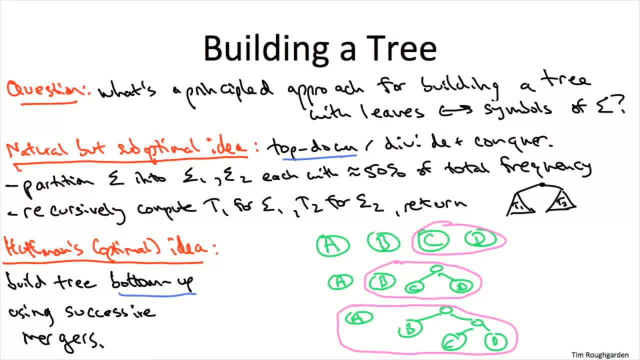 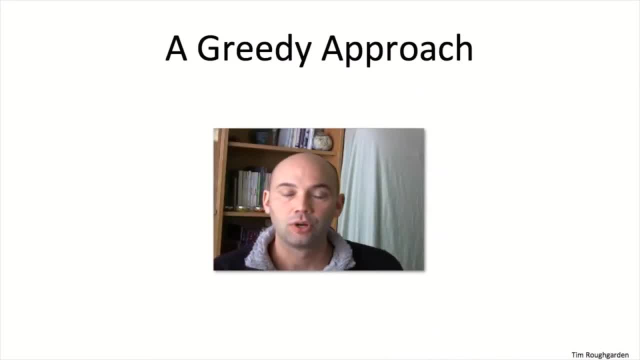 lopsided tree we were using in the previous video as a running example. So let me explain what I hope is clear and what is maybe unclear. at this juncture, I hope what's intuitively clear is that the bottom-up approach is a systematic way. 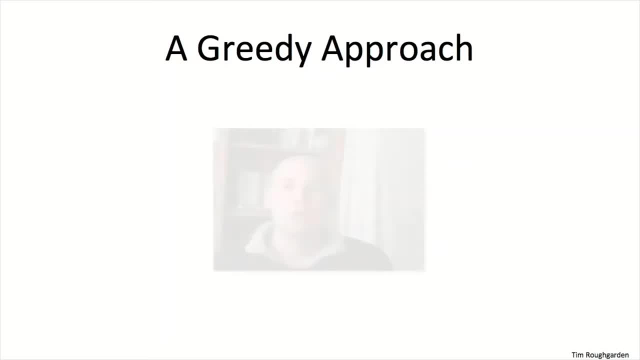 to build trees that have a prescribed set of leaves. So what do we want? We want trees whose leaves are labeled with the symbols of the alphabet sigma. So if we have an alphabet with n symbols, we're going to start with just the n leaves. 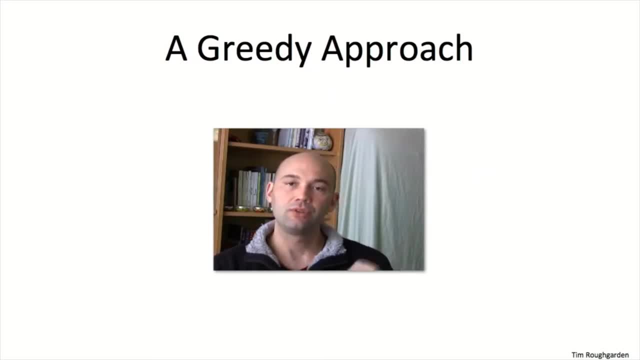 What does a merger do? Well, it does two things. First of all, it introduces a new internal node, an unlabeled node, And secondly, it takes two of our old subtrees and fuses them into one, merges them into one. 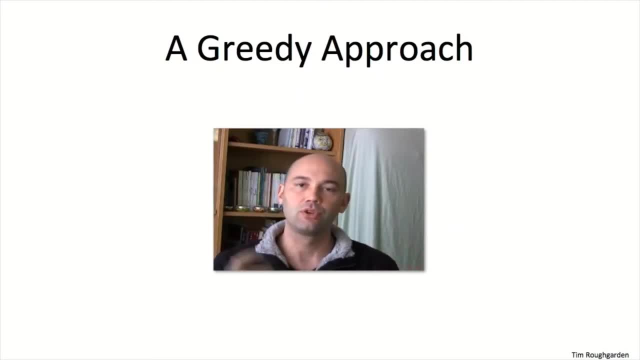 We take two subtrees, we make one the left child of this new internal node, the other the right child of this new internal node. So that drops the number of subtrees we're working with by one. So if we start with the n leaves and we do n minus one successive mergers. 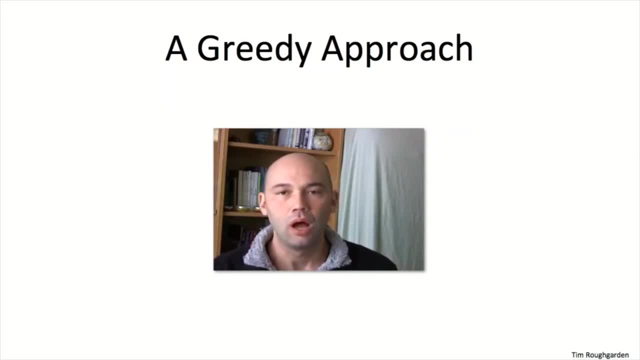 what happens? Well, on the one hand, we introduce n minus one new unlabeled internal nodes And on the other hand, we construct a single tree, And the leaves of this tree that we get are in one to one correspondence with the alphabet letters as desired. 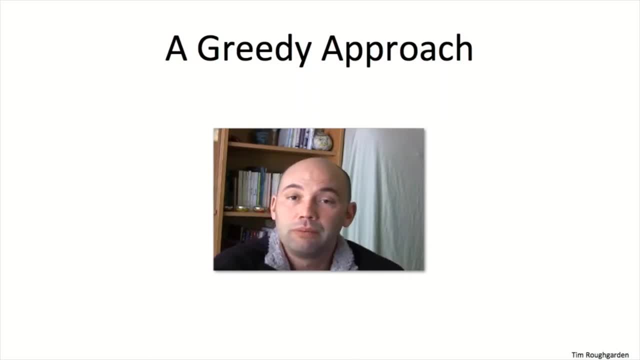 Now, what I don't expect you to have any intuition for is: what should we be merging with what and why? Forget about you know how do we get an optimal tree at the end of the day? I mean, even just if we wanted to design a greedy algorithm. 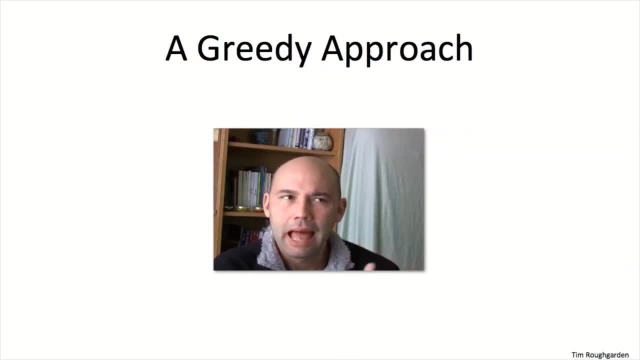 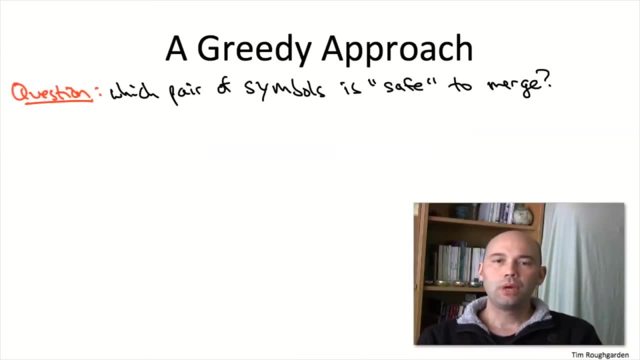 if we just wanted to make a myopic decision that looks good right now, how would we even do that? What's our greedy criterion that's going to guide us to merge a particular pair of trees together So we can reframe this quandary in the same kind of question we asked for? 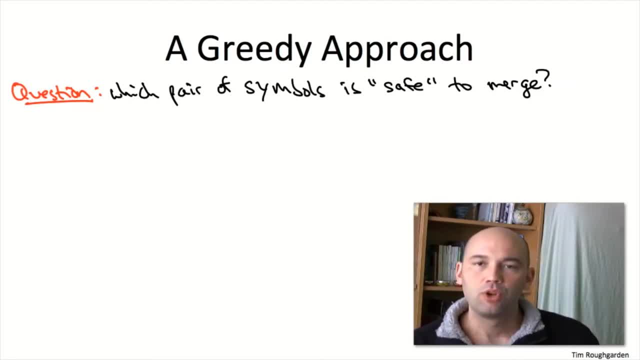 minimum cost spanning trees, and really more generally, with greedy algorithms, When you're making irrevocable decisions, what strikes fear in your heart is that this decision will come back and haunt you later on. You'll only realize at the end of the algorithm that you made some horrible. 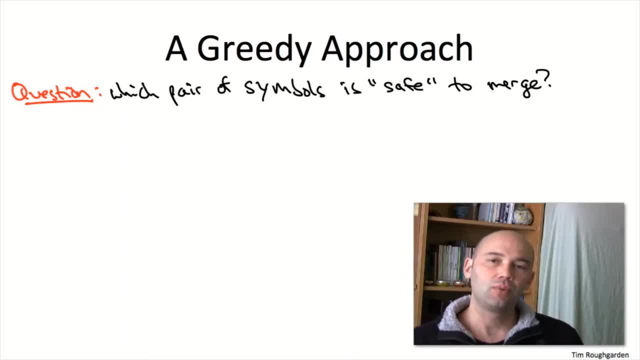 mistake early on in the algorithm. So, just as for MSTs, we ask you know, when can we be sure that including an edge irrevocably is not a mistake, is safe in the tree that we're building Here? we want to ask you know, we have to do a merger. 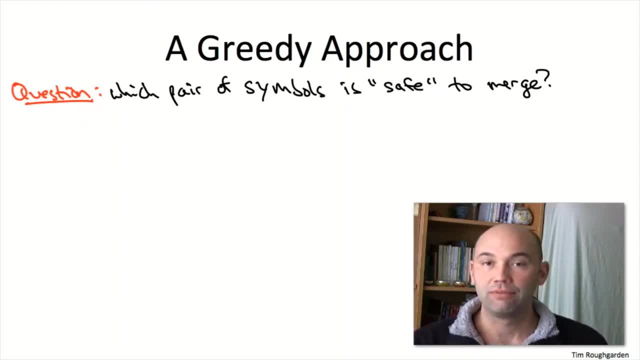 We want to do successive mergers, And how do we know that a merger is safe, That it doesn't prevent us from eventually computing an optimal solution? Well, here's the way to look at things that will at least give us an intuitive conjecture for this question. 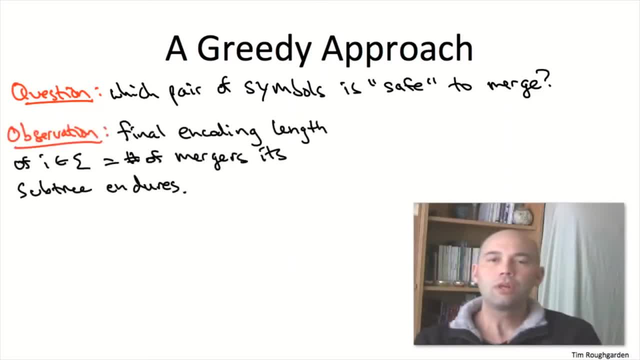 We'll save the proof for the next video. So what are the ramifications when we merge two subtrees each containing a collection of symbols? Well, when we merge two subtrees, we introduce a new internal node which unites these two subtrees under them. 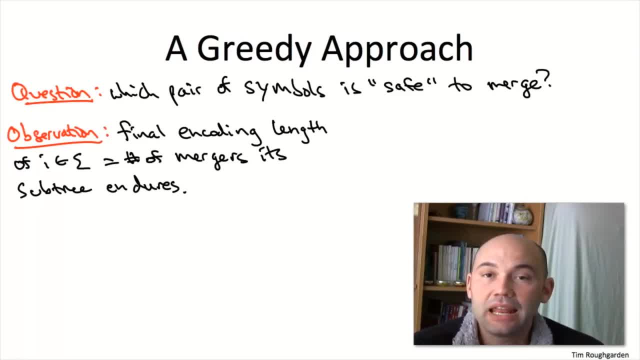 And if you think about it, at the end of the day, in the final tree, this is yet another internal node that's going to be on the root to leaf path for all of the leaves in these two subtrees, That is, if you're a symbol and 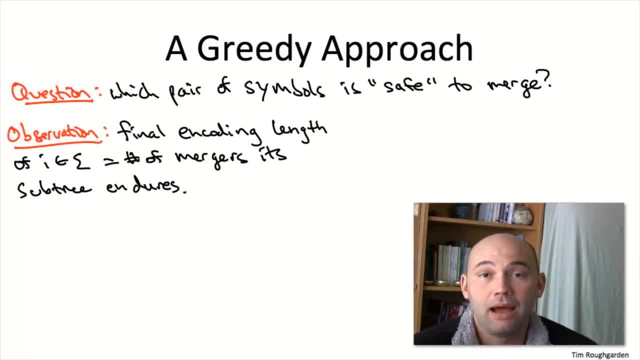 you're watching your subtree get merged with somebody else. you're bummed out. You're like man. that's another bit in my encoding. That's yet one more node I have to pass through to get back to the root. I think this will become even more clear if we look at an example. 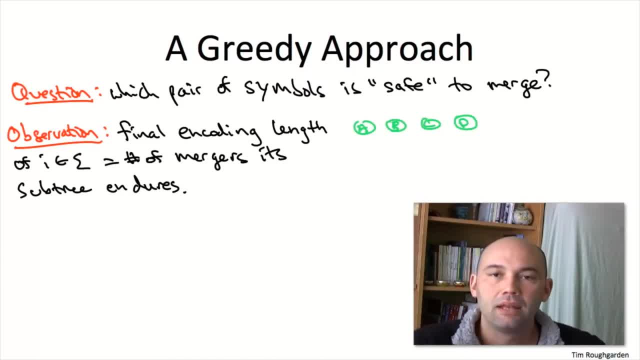 So naturally we'll use our four symbol alphabet- A, B, C, D, And initially, before we've merged anything, each of these is just its own leaf- A, B, C, D, So there's no internal nodes above them. 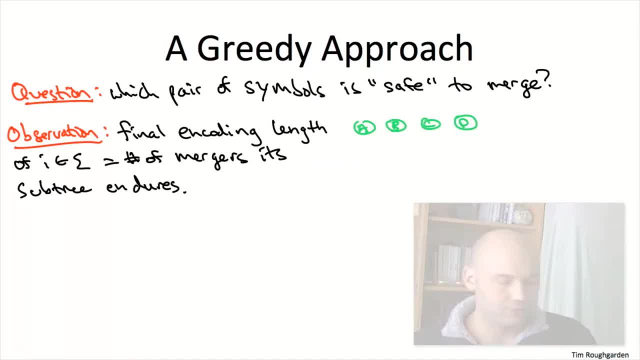 In a sense, everybody's encoding length at the beginning is zero bits. So now imagine we merge C and D, We introduce a new internal node which is the common ancestor of these two leaves And as a result, C and D are bummed out. 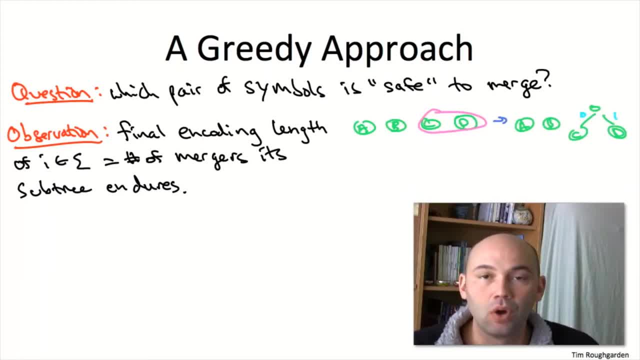 They say: well, there's one bit that we're going to have to incur in our encoding length. There's one new internal node we're always going to have to pass through on route back to the root of the eventual tree. Now suppose next we merge B with a sub-tree containing both C and D. 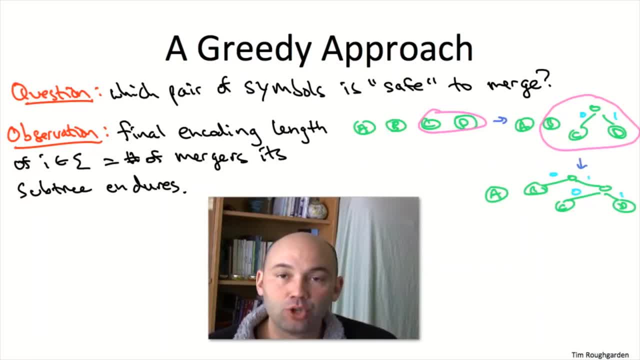 Well, everybody but A's bummed out about, about this merger, because we introduce another internal node and it contributes one bit to the encoding of each of B, C and D. It contributes an extra 1 to the encoding of C, D and D. 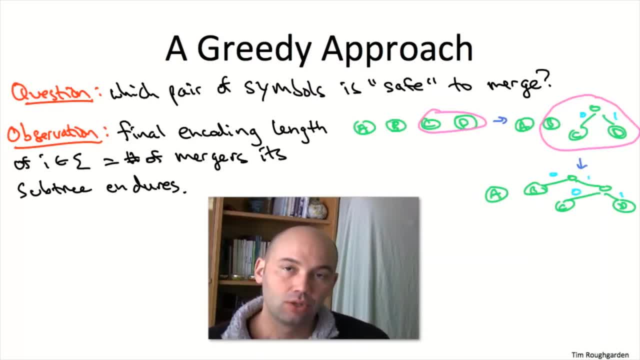 Okay, So you're bummed. It's not a bummer. Okay, C and D, and it contributes a zero to the encoding of B, So all of their encodings in some sense get incremented, go up by one compared to how things were before. 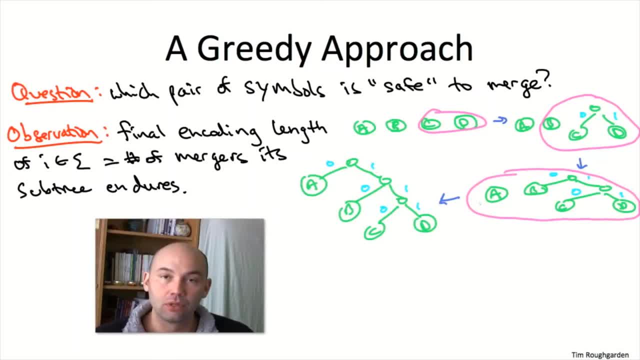 Now, in the final iteration, we have to merge everything together. We have no choice. There's only two subtrees left, So here everybody's encoding length gets bumped up by one, So A finally picks up a bit, namely zero to encode it. 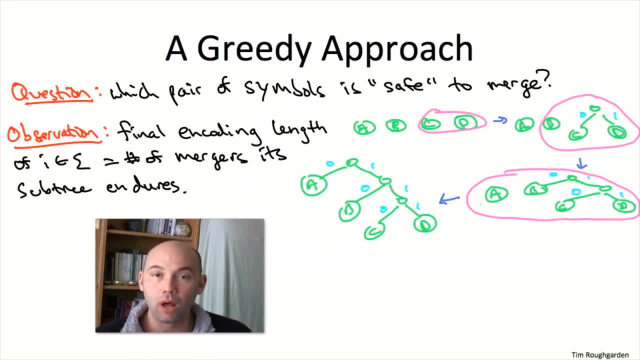 And B, C and D each get pick up an additional bit of one which is prepended to their encodings. thus far, And in general, what you'll notice is that the final encoding length of a symbol is precisely the number of mergers that its subtree has to endure. 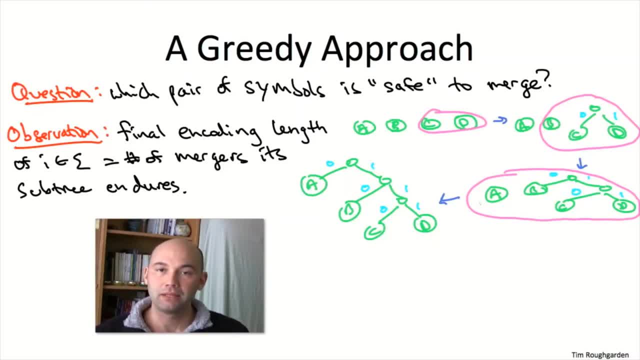 Every time your subtree gets merged with somebody else, you pick up another bit in your encoding, And that's because there's one more internal node that you're going to have to traverse on route to the route of the final tree, In this example, the symbols C and D. well, 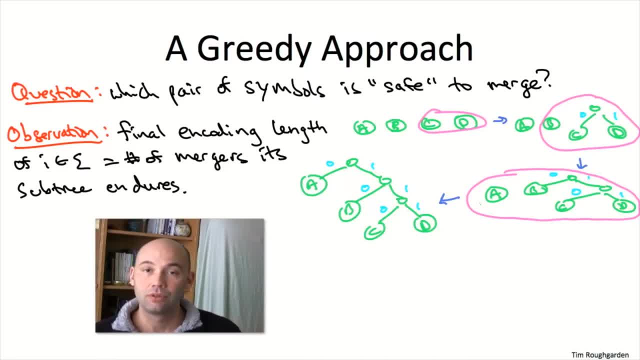 they got merged with somebody else in each of the three iterations, So they're the two symbols that wind up with an encoding length of three. The symbol B: it didn't get merged with anybody in the first iteration, only in the second two. 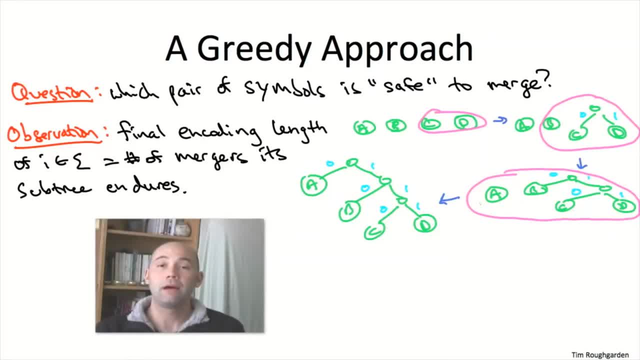 That's why it has an encoding length of two. So this is really helpful. So this lets us relate the operations that our algorithm actually does, namely mergers, back to the objective function that we care about, namely the average encoding length. Mergers increase the encoding lengths of the participating symbols by one. 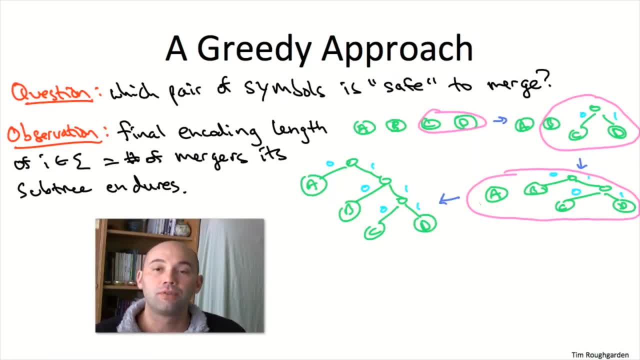 So this allows us to segue into the design of a greedy heuristic for how to do mergers. Let's just think about the very first iteration. So we have our N original symbols and we have to pick two to merge. And remember the consequences of a merge is going to be an increase in the encoding. 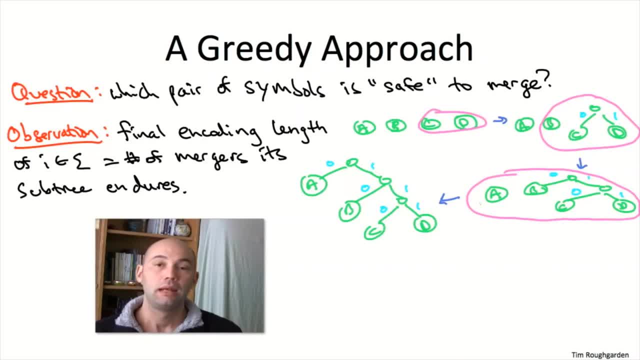 length by one bit. of whichever two symbols we're going to pick Now, what we want to do is minimize the average encoding length with respect to the frequencies that we were given. So which pair of symbols are we the least unhappy to suffer an increment to their? 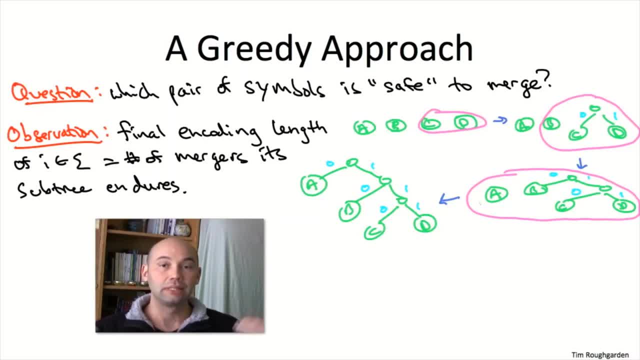 encoding length. What's going to be the symbols that are the least least frequent? That's going to increase our average coding length by the least. So that's the green emerging heuristic. Something's got to increase. Pick the ones that are the least. 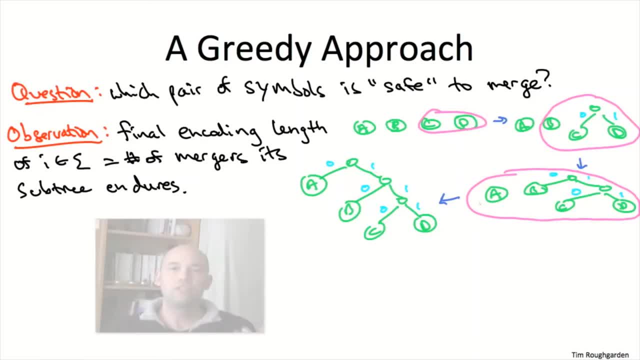 frequent to be the ones that get incremented. So that seems like a really good idea of how to proceed in the first iteration. The next question is: how are we going to recurse? So I'll let you think about that in the following quiz. 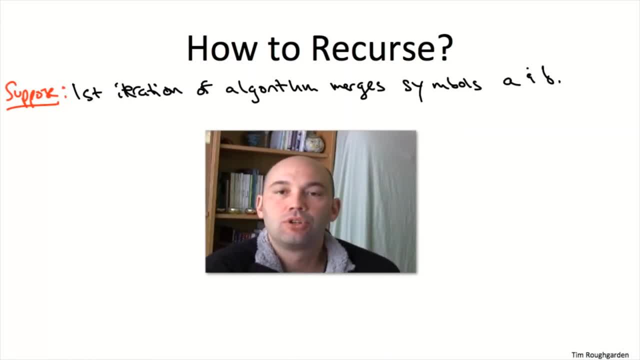 So let's agree that the first iteration of our greedy heuristic is going to merge together the two symbols that possess the lowest frequencies. Let's call those two symbols little a and little b. The question is then: how do we make further progress? What do we do next? Well, one thing that would be really nice. 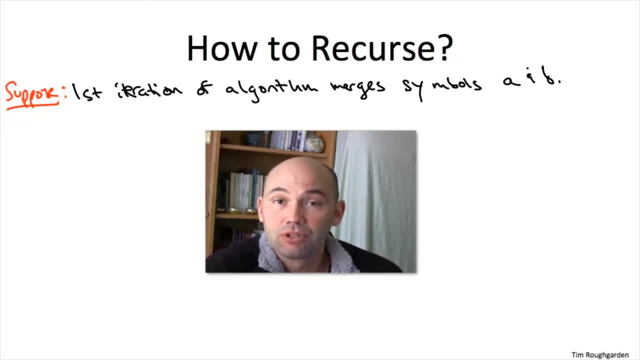 is if we could somehow recurse on a smaller sub-problem. Well, which smaller sub-problem? Well, what does it mean that we merge together the symbols a and b? Well, if you think about it, in the tree that we finally construct by virtue of us merging a and b, we're forcing the 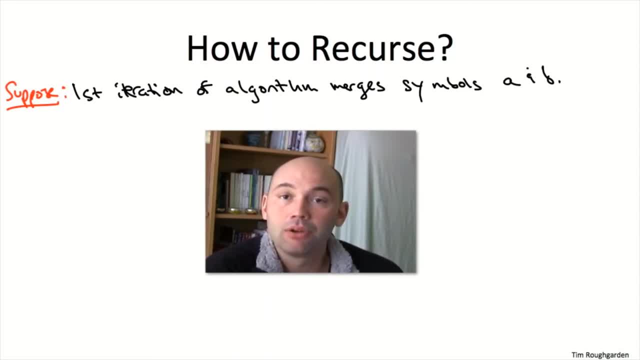 algorithm to output a tree in which a and b are siblings, in which they have exactly the same parent. So what does it mean for the encoding that we compute that a and b are going to be siblings with the same parent? It means their encodings are going to be identical, save for the lowest order. 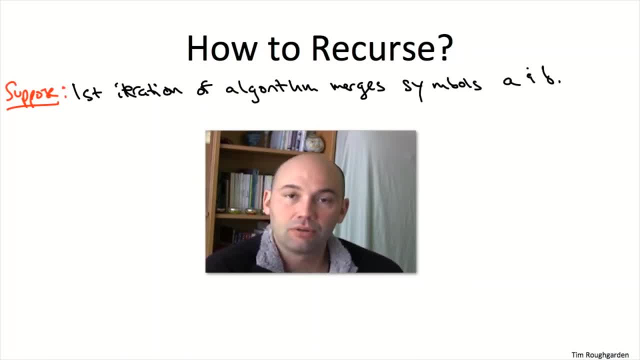 bits. So a will get encoded with a bunch of bits followed by a zero. b will be encoded by exactly the same prefix of bits followed by a one. So they're going to have almost the same encoding. So for our recursion let's just treat. 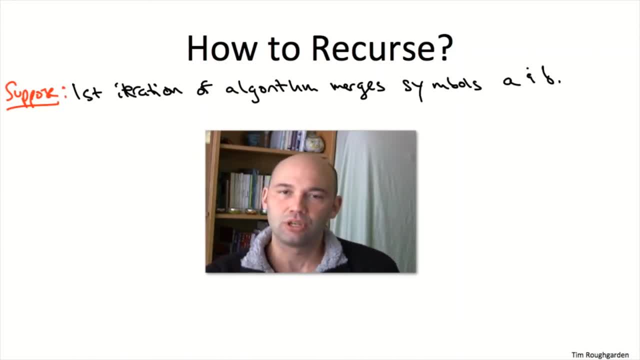 them as the same. So let's introduce a new meta-symbol- let's call it a- b- which represents the conjunction of a and b, So it's meant to represent all of the frequencies of either one, all of the occurrences of either one of them. 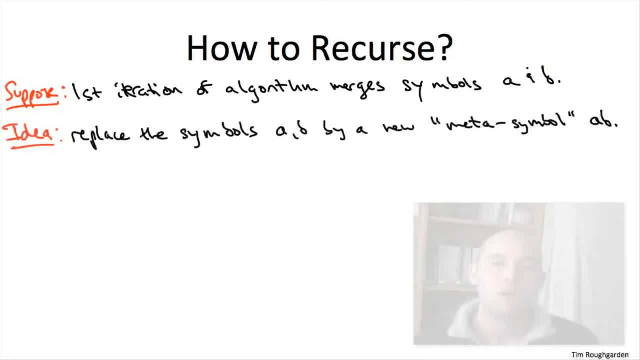 But remember, the input to the computational problem that we're studying is not just an alphabet, but also frequencies of each of the symbols of that alphabet. So my question for you is: when we introduce this new meta-symbol a, b, what should be the? what should be the? 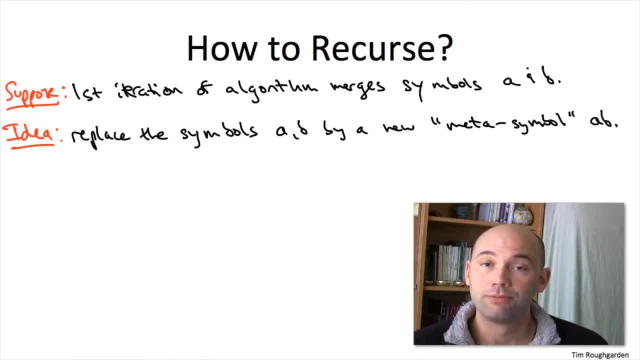 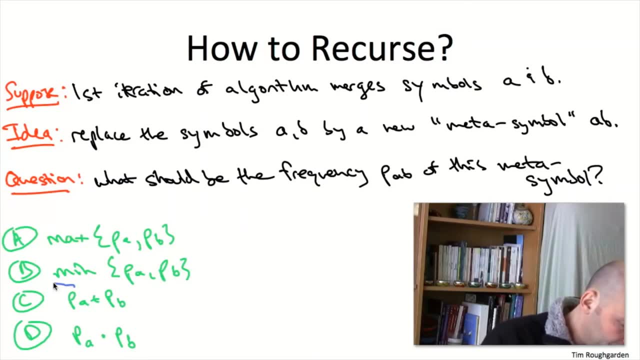 frequency that we define for this meta-symbol. All right, so hopefully, your intuition suggested answer c- that for this recursion to make sense, for it to conform to our semantics of what this merging does, we should define the frequency of this new meta-symbol to be the sum of the 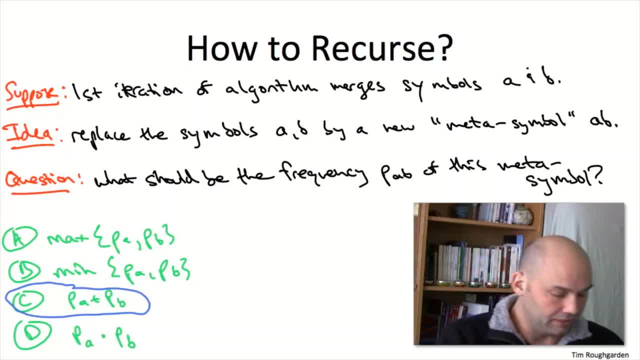 frequencies of the two symbols that it's replacing. That's because, remember, this meta-symbol- a- b, is meant to represent all occurrences of both a and b, So it should be the sum of the frequencies of the two symbols. So I'm now ready to formally describe. 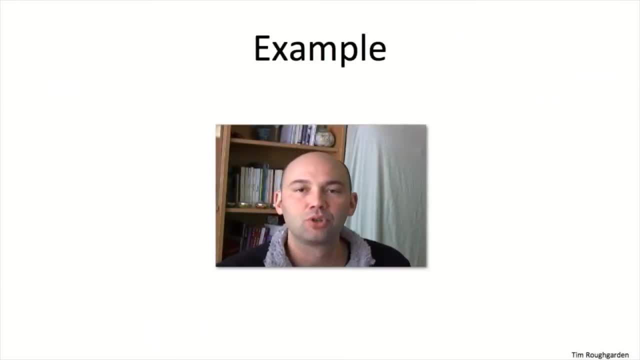 Huffman's Greedy Algorithm. Let me first describe it on an example, and then I think the general code will be self-evident, So let's just use our usual example. So we're going to have letters a, b, c, d. 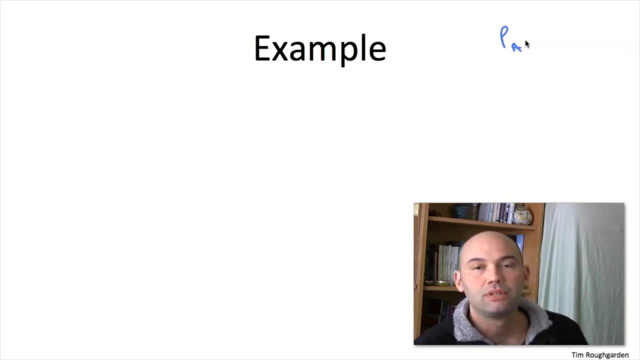 with frequencies 60,, 25,, 10, and 5.. So we're going to use the bottom-up approach. So we begin with each symbol just as its own node: a, b, c, d, i b c, d, i b c d. 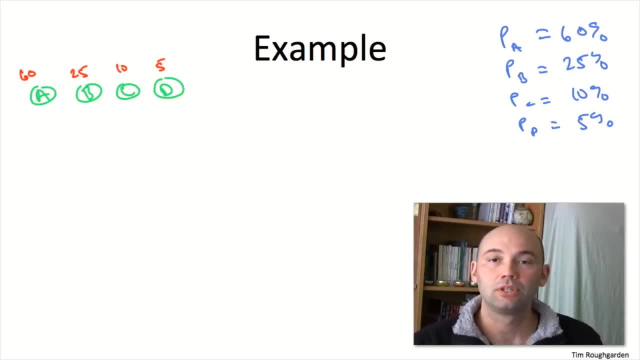 I'm annotating in red the frequencies 60,, 25,, 10, 5.. The greedy heuristic says initially we should merge together the two nodes that have the smallest frequencies, So that would be the c and the d with their frequencies of 10 and 5.. Now, based on the idea of the last slide, 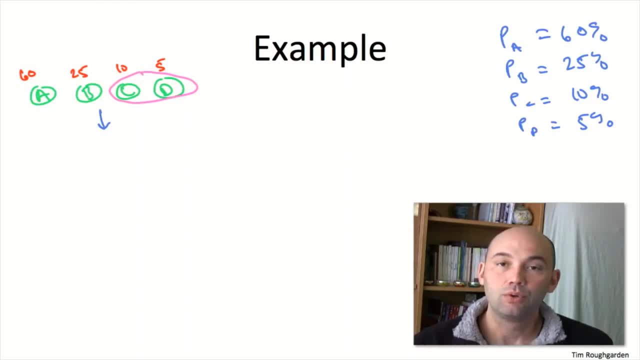 when we merge c and d, we replace them with a meta-symbol, cd, whose frequency is the sum of the frequencies of c and d, namely 15.. Now we just run another iteration of the greedy algorithm, meaning we merge together the two nodes, the two symbols that have the smallest frequencies. 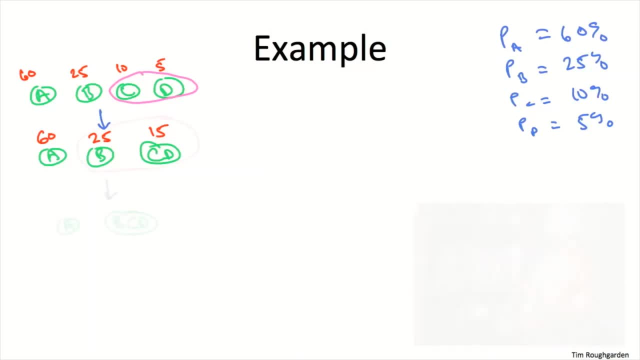 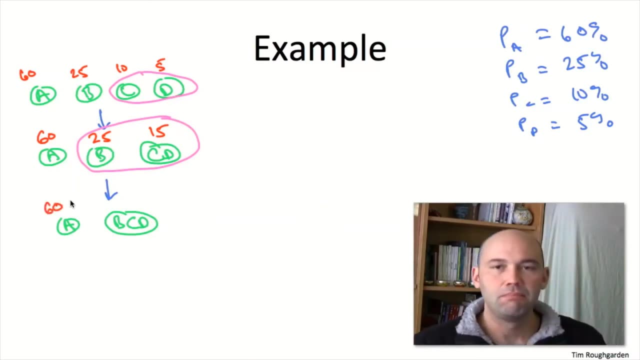 So this is now b 25, and cd 15.. So now we're down to just two symbols: the original symbol a, which still has frequency 60, and the in some sense meta-meta-symbol bcd, who is now cumulative frequency is 40. 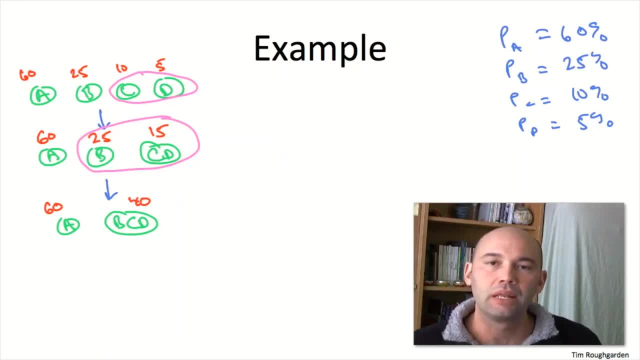 So when we're down to two nodes, that's going to be the point in Huffman's algorithm where we hit the base case and the recursion begins to unwind. So we have two symbols to encode. There's pretty much only sense, one sensible way to do it. One is a zero and one is a one. 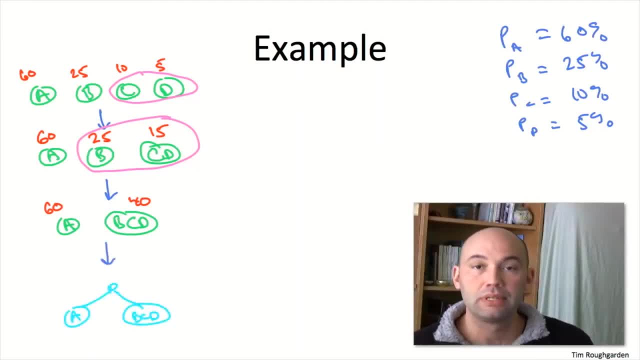 So at this point the final recursive call just returns now a tree with two leaves corresponding to the symbols a and bcd, And now, as the recursion unwinds, we in effect undo the mergers. So for each merge we do a corresponding split of the meta-node and we replace 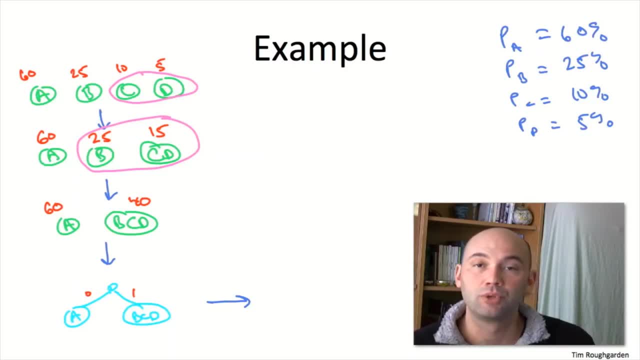 that with an internal node and then two children corresponding to the symbols cd are merged to make that meta-node. So for example, when we want to undo the merge of the b and the cd, we take the node labeled bcd and we split it into two. 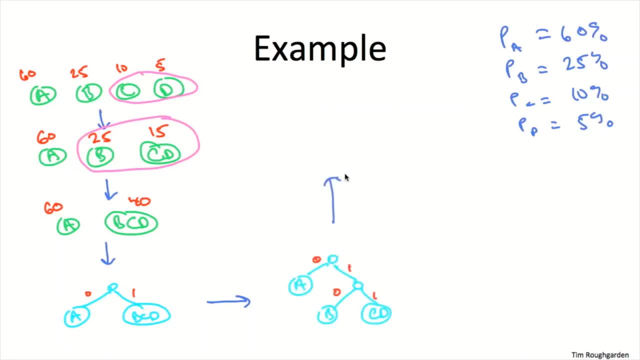 the left child being b, the right child being cd, So the original outermost call, what it gets from its recursive call, is this tree with three nodes and it has to undo its merger. it merged c and d, So it takes the leaf labeled with the symbol cd and splits it into two. 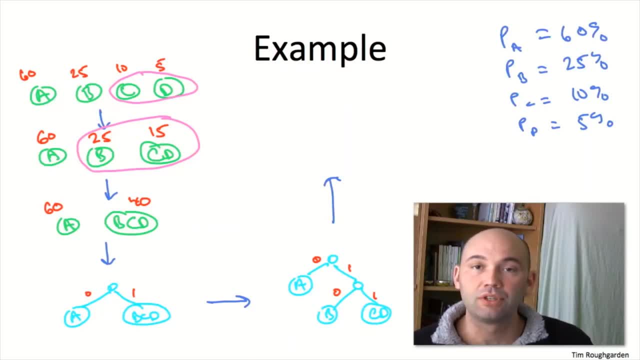 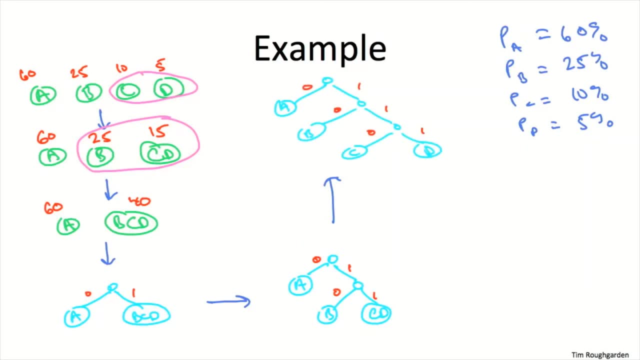 It replaces it with a new unlabeled internal node- Left child c, right child d. So how does the algorithm work in general? Well, just as you'd expect, given the discussion on this concrete example I'm going to take as the base case when the alphabet has just two symbols. 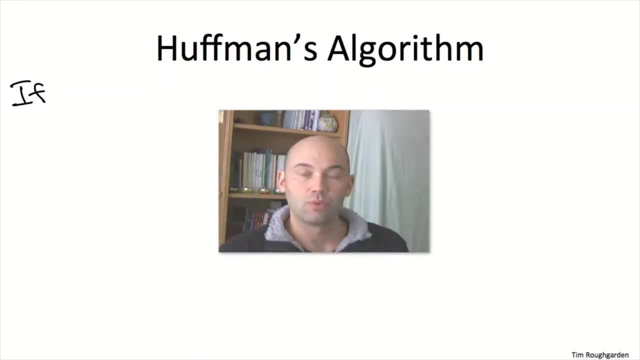 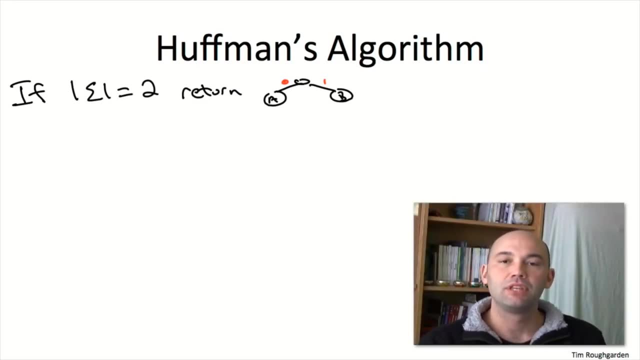 In that case, the only thing to do is encode one with a 0, the other with a 1.. Otherwise, we take the two symbols of the alphabet that have the smallest frequencies. You can break ties arbitrarily, it's not going to matter. it's going to be optimal either way. 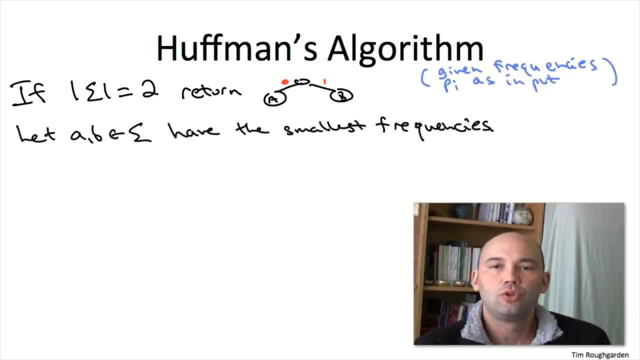 We then replace these two low frequency symbols, a and b, with a meta symbol, ab, intended to represent both of them in some sense. As we just discussed with those semantics, we should be defining the frequency of the meta symbol ab as the sum of the frequencies of the symbols that it 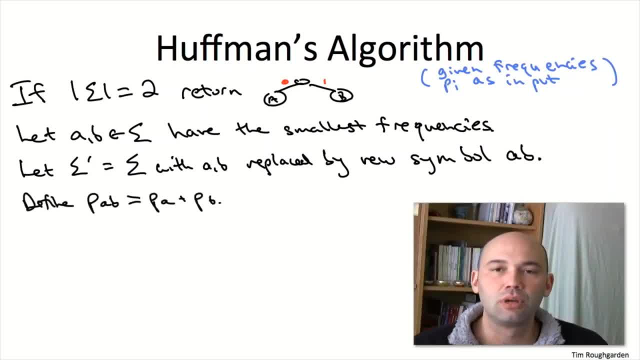 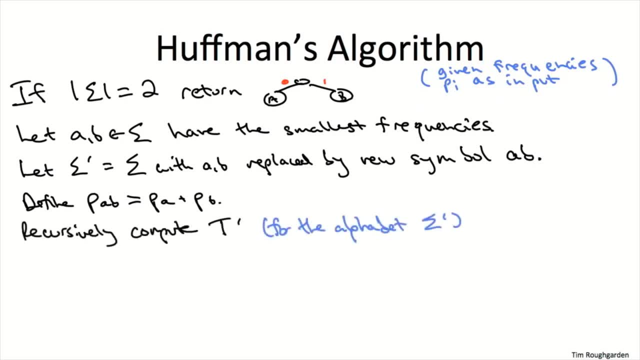 comprises. We now have a well-defined, smaller subproblem. It has one fewer symbol than the one we were given, so we can recursively compute a solution for it. So what the recursive call returns is a tree whose leaves are in one-to-one correspondence with sigma prime. 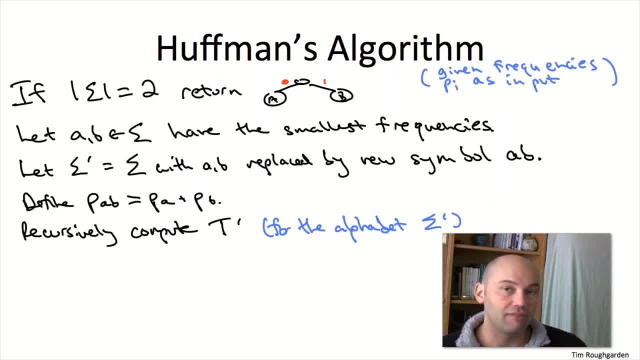 That is, it does not have a leaf labeled a, it does not have a leaf labeled b, it does have a leaf labeled ab. So we want to extend this tree t prime to be one whose leaves correspond to all of sigma, And the obvious way to do that is to split the leaf labeled ab. replace that. 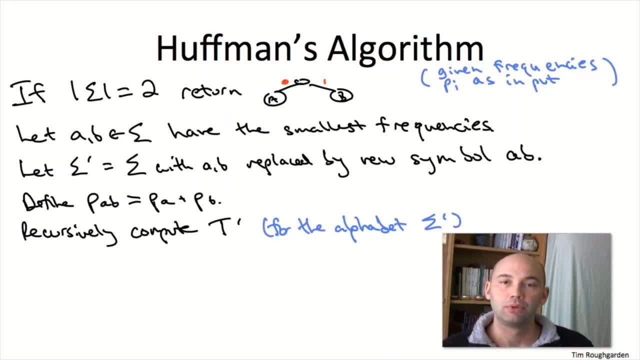 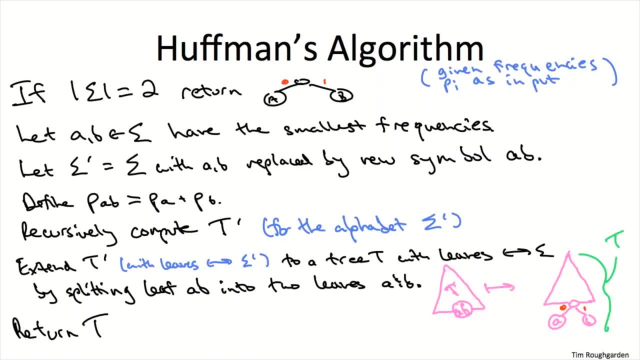 with a new internal unlabeled node with two children which are labeled ab. The resulting tree capital T with leaves in correspondence to the original alphabet sigma, is then the final output of Huffman's algorithm. As always with a greedy algorithm, we may have intuition. it may seem like a good. 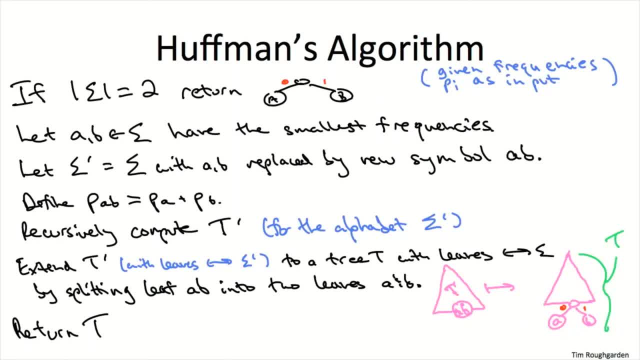 idea, but we can't be sure without a rigorous argument. That is the subject of the next video.